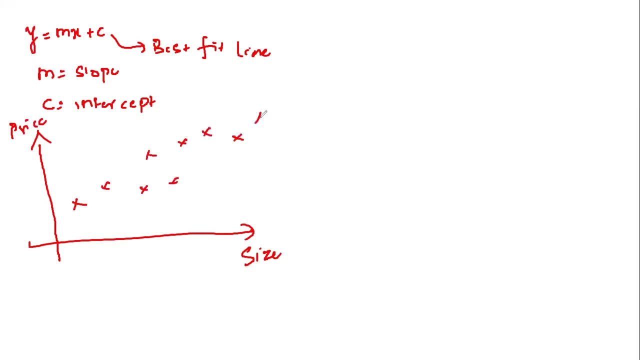 So some of the points will be somewhere populated like this: you know, and what we are actually considering, or what we are trying to implement by using a regression line, regression algorithm- is basically that we'll try to create a best fit line such that this best fit line- what you know, it will indicate that for my future size. 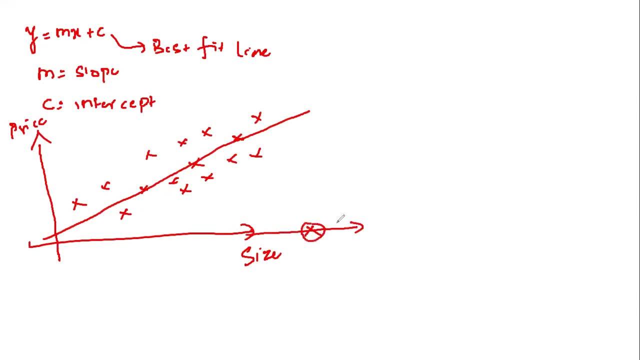 suppose for this particular size i want to find out what may be the price of the particular house, then what i can do is that i can actually point to this particular point over here and i can try and find out the price value, and i'll be able to determine the price with the help of this best. 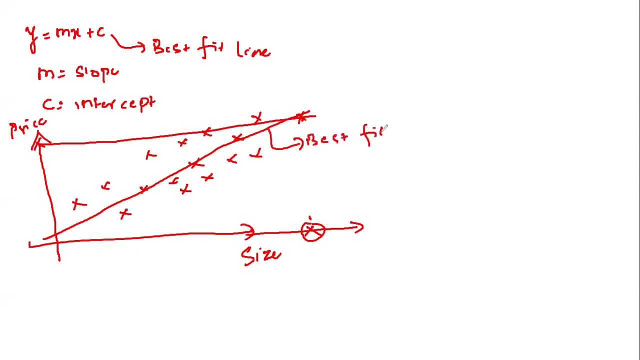 fit line. so this is my best fit line and, as discussed, this best fit line is basically indicated by the equation: y is equal to mx plus c. now what does this component mean? that is my m value and my c value. guys always remember, whenever your size is zero and your price is zero, 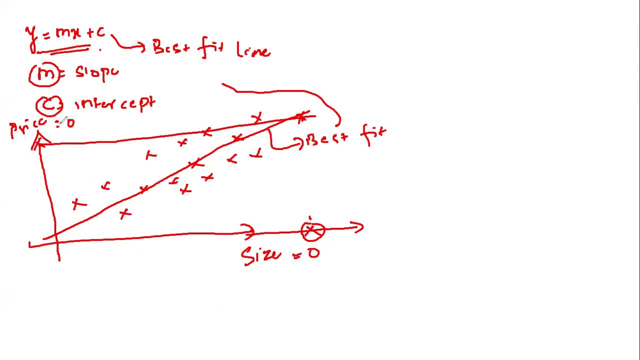 right, or whenever your size is zero. right, not price is zero, i'll just cut this okay- whenever your size is zero. now over here, when i consider this size, i am basically considering that my x value is zero. so this from this equation, my, if my x value is zero. so if my x value is zero, 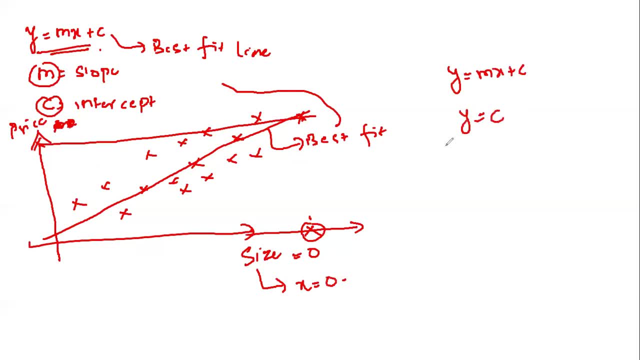 uh, if i equate, in this particular equation, my y will basically be c, so my y will basically be the c, which is the constant or the intercept, and this basically indicates that when my size is zero at this particular point, where does my price actually point to the price of the house? and when my size 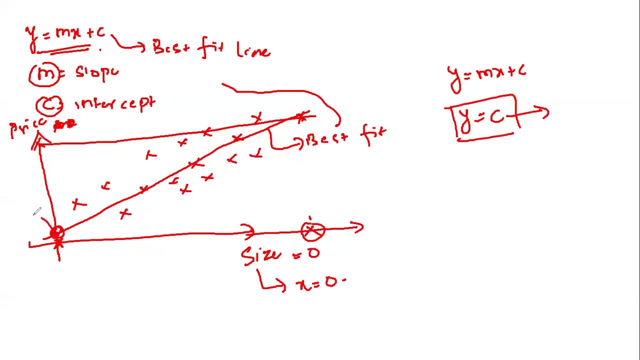 is zero, it is going to be c. okay, so this particular point in this particular equation is basically my c, which is my intercept. so when my size is zero, and what is the point that i have in the y-axis for the price? that is the point that is called as c. the other thing that i want to discuss is about m. 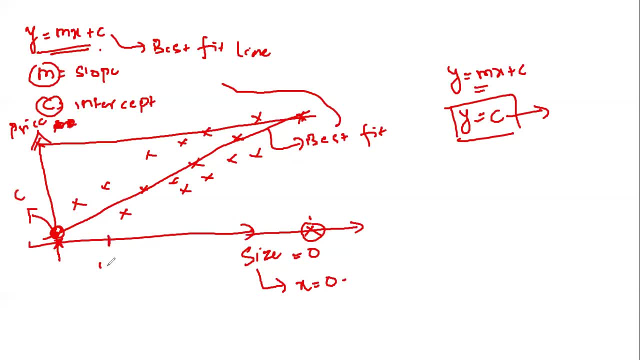 this m basically indicates that suppose, uh, over here i have something like thousand square, okay, thousand square meter, uh, thousand square feet, and here i have, suppose, 1100 square feet right now within this unit change, suppose, if i'm considering that 100 meter is my unit change in my. 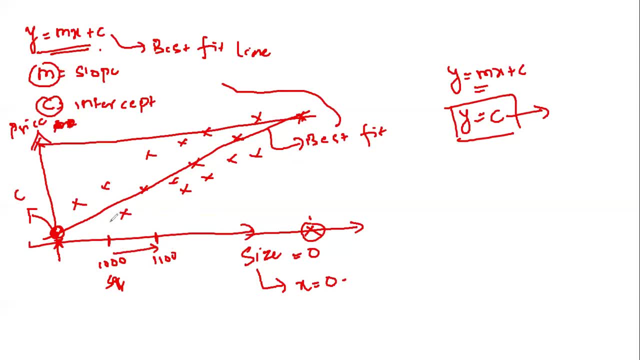 x-axis within this unit change. with this unit change, what is the change in your best fit value? what is the change of the price? that we are actually considering it as a slope. so this particular slope is basically indicating that with the unit change in my x-axis, that means my size. 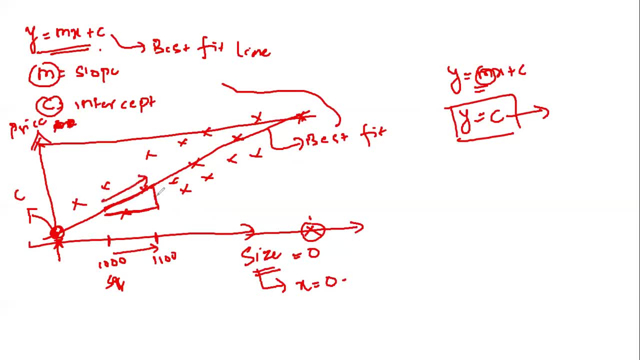 what will be the change in your y-axis. you know, and that is what we are trying to find out now. now, the other way that you may be thinking, that, how can we think of a best fit line, you know, in this particular equation? see, one way is that i can draw multiple best fit line, you know. 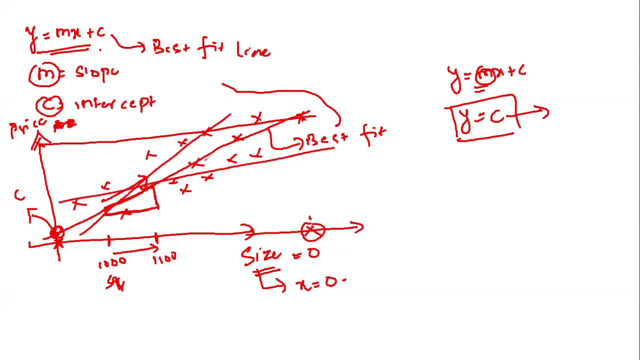 multiple best fit line like this, and what i should try to do is that i should try to minimize this distance, you know, minimize this particular distance or this particular error such that if i do the summation of all the error, it should be minimal. right, it should be minimal. so this: 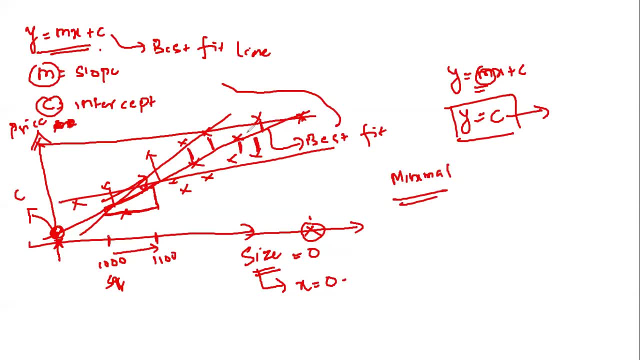 particular error, we should try to find out the summation of all the error and whichever best fit line gives us the minimal error. that value will will basically indicate or give me the slope value, that is, m, and some value as c, c which is my, which will be my intercept. now again, i'll just clear this. 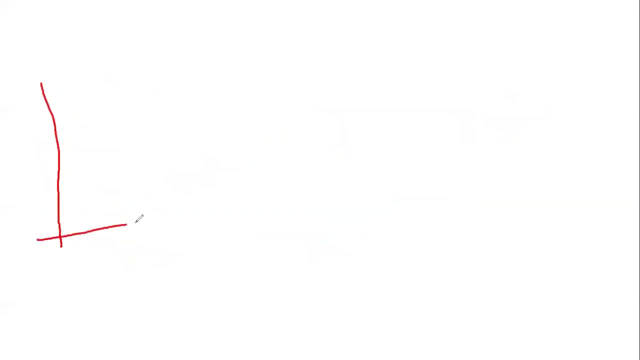 diagram and just try to explain you properly. now you see this. oops, sorry, now suppose i have this. okay, i have this. uh, x and y value. suppose my x is basically my size and y is basically my price and i have a lot of points that is getting populated, you know now, from this i found out that best fit line is this one. 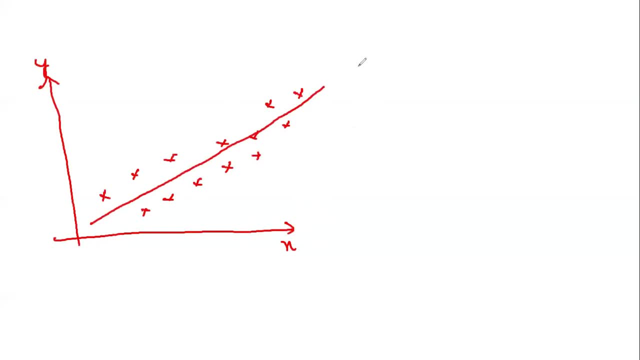 okay, now what we should consider while selecting the best fit line. i will define a function which is called as cost function. again, guys, this cost function is very, very important. okay, this cost function is also a basic thing that we'll also be learning in deep learning, so it is very important. 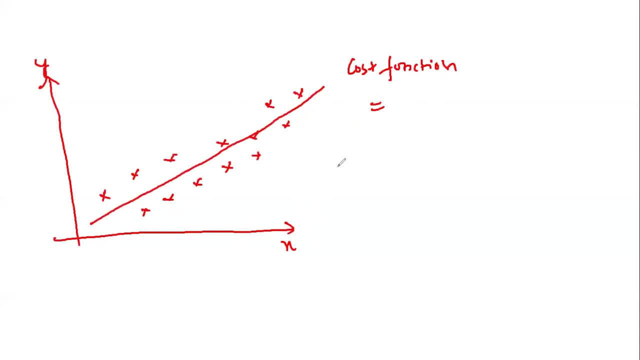 to understand this. so make sure that you watch this particular video till the end. so now this cost function can basically be indicated that, as we said, that the distance between the best fit point- that is, this- and my real point should be minimal. so i can write an equation. 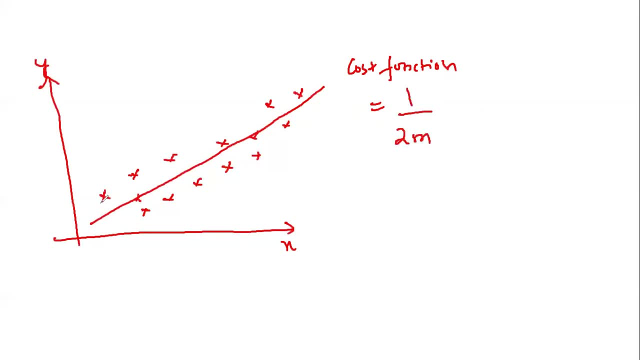 saying as 1 by 2 m. m basically means that it is the number of points, all the points you know, with respect to the x and y axis. 1 by 2 m, i'll say summation of i is equal to 1 by m 1. 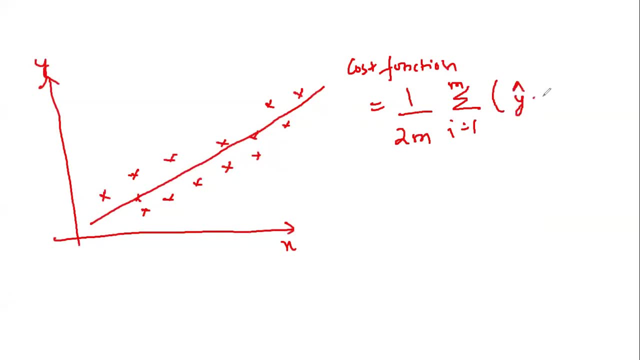 to m, and then i will write it as y hat minus y whole square, and this is what i'm going to write it down now. you know that my y hat will basically be indicated by: y is equal to mx plus c. this points that i have over here, right, this is basically my y hat. you know, this is my y hat, the points that you. 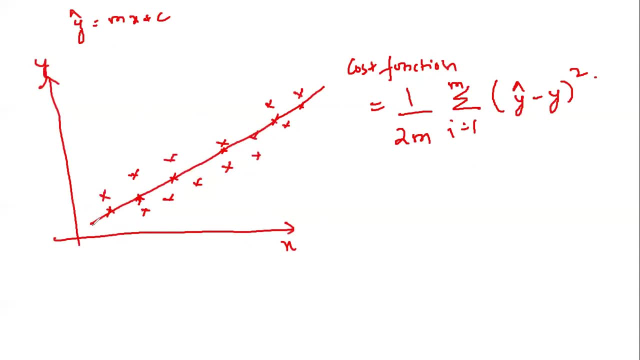 find out or that you predict in a best fit line is basically your y hat, and this y basically indicates the points you know. it indicates the real points. so we should try to minimize this error. we should try to minimize this error and while minimizing whichever will, whichever best fit line gives you, 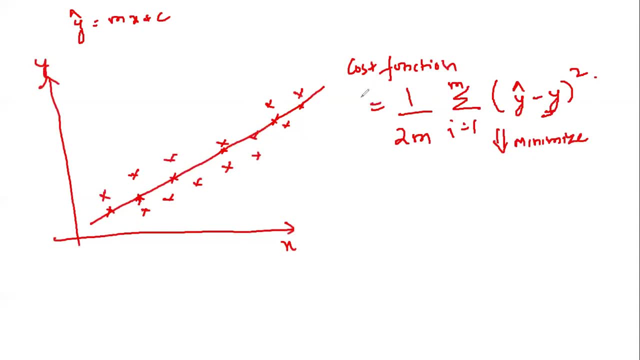 the minimum error, that is selected as the best fit line. but now the next question rises: that just by using this equation, how do i find out the best fit line? because i can have multiple best fit lines, right, i can have a lot of best fit lines, you know. and then from that i have 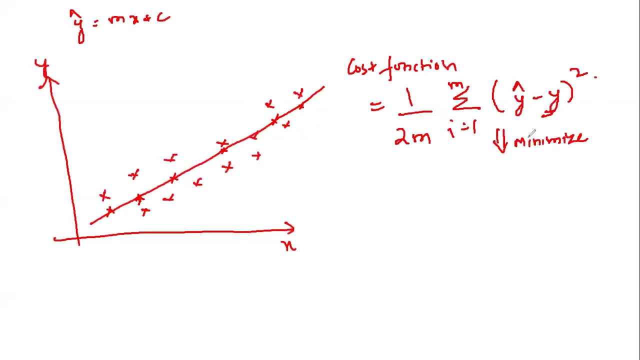 to compute all the summation and then try to find out what is the minimal value. that will not exactly work. you know that is actually that will actually take more amount of time and which will unnecessarily waste your amount of processing power and amount of processing itself. you know. 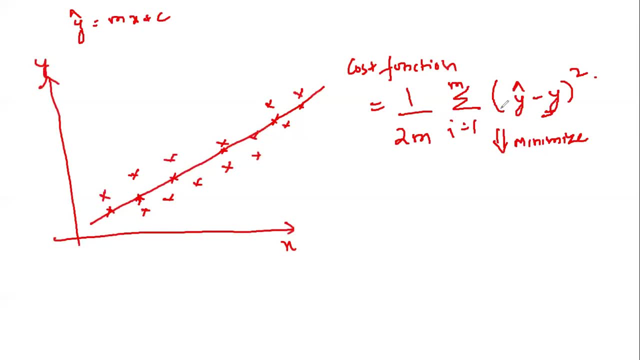 we can't just select million number of lines and try to find out the cost function. instead, i'll just show you a more efficient way. so to begin with, i'm going to give you an example again. so suppose i am considering x and y. okay, so this is my x, okay? 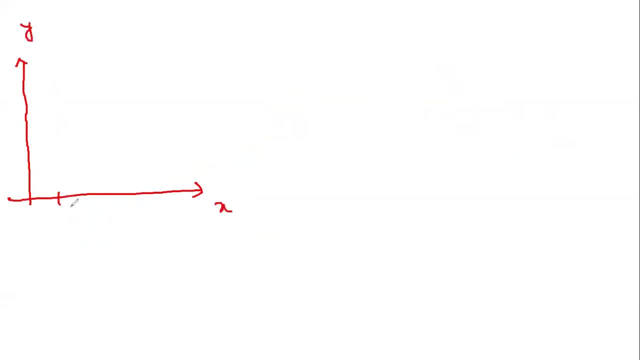 and this is my y, and suppose, uh, this values, i have like one, two, three and four right, and similarly i have over here one, two, three, four. now suppose let me consider some points over here. suppose my first point, my y point, is basically when my x value is one, my y value is also one. so i'll draw my first. 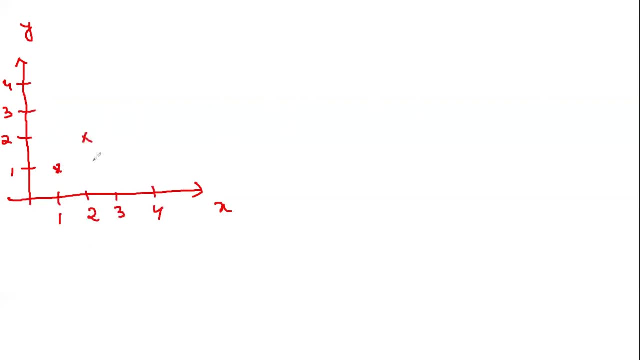 point over here. my x value is two, my y value will also be two. my second point: my x value is three, my will also be three. suppose these are my three points. okay, and now this is my data. this is my real data. okay, and this real data is basically given by the equation: y is equal to x because 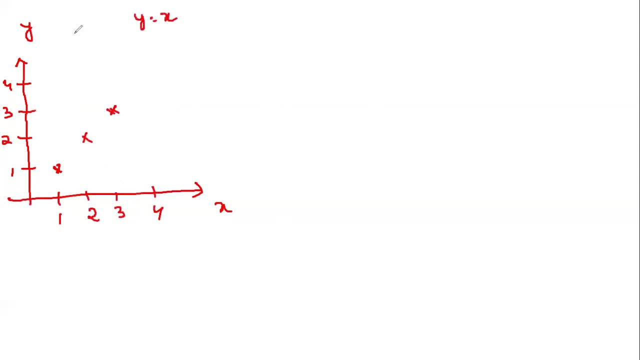 when i'm saying my x value is one, my y value is one. now, the next thing is that i need to find out my best fit line, you know, for this particular point. so i'll write the equation as: y is equal to mx plus c. okay, now let me consider that my c value is zero. okay, the reason why i'm telling. 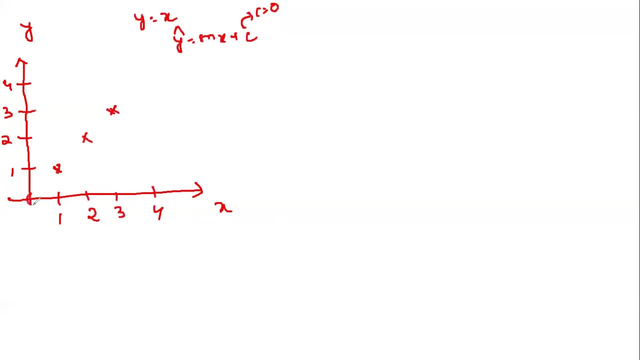 you. that is because you can see that in this particular point that i'm drawing a line through this particular point. so i'm going to draw a line through this particular point and i'll consider that that c value passes through the origin. you know the origin. when my x value is zero, my y value 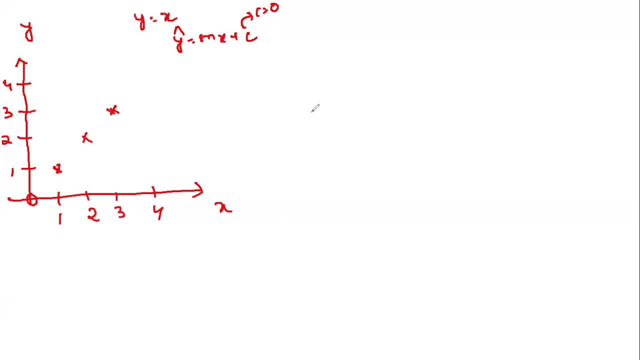 will be zero. right. and again, there is a reason why i'm making it a c is equal to zero, because i'm going to draw a diagram over here which, uh, if i make c is equal to 0, then i will be able to draw a 2d diagram. if not, if i consider c is equal to with some other value, then i have to basically draw. 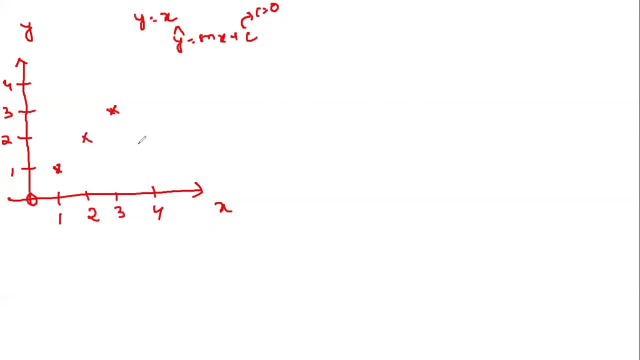 it over here. okay, so i'm considering the c value as 0, indicating that it passes through the origin. okay, when my x value is 0 and my y value is 0.. so when i make the c value as 0, my new equation is: 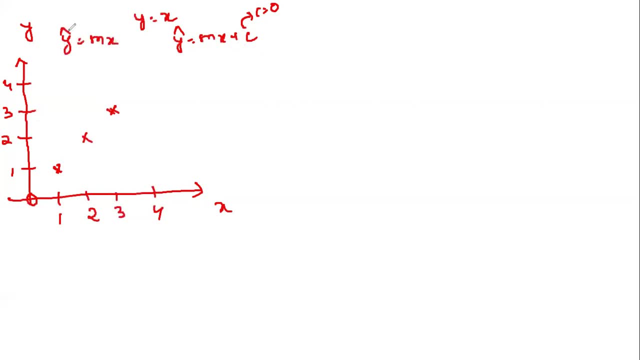 something like y is equal to mx. now this y hat is basically indicating my best fit line. so for x is equal to 1, for x is equal to 1. let me equate x is equal to 1 and try to find out my y hat value. 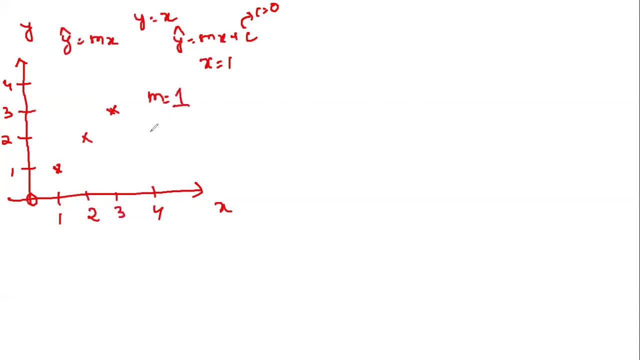 and let me consider that my m slope. initially i'm just initializing my m as 1. okay, so when my m is 1? so let me just equate it over here. okay, so when my m is 1. so this basically indicates that my y hat is basically 1 multiplied by 1.. 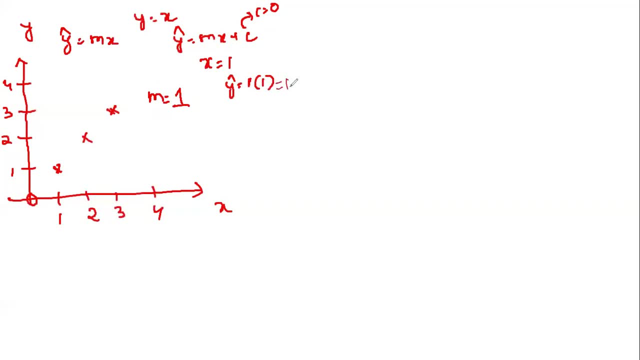 let me just write it in a lighter format. so y, y hat will be actually 1, right? so my first point after 0, my best fit line, will pass through this y hat. okay, so this particular point also has y hat and this particular point also has y. now, for my x is equal to 2. what will be my y hat? 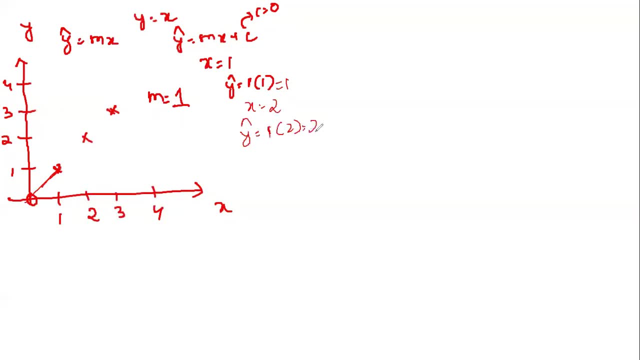 you know that my slope is 1 and my x value is 2, so it will be 2.. so then again this line gets extended and gets passed through this particular point. similarly, y hat when my value is 1 and my x value is 3, because my x value is 3 and this particular point is 3, then again my y hat will. 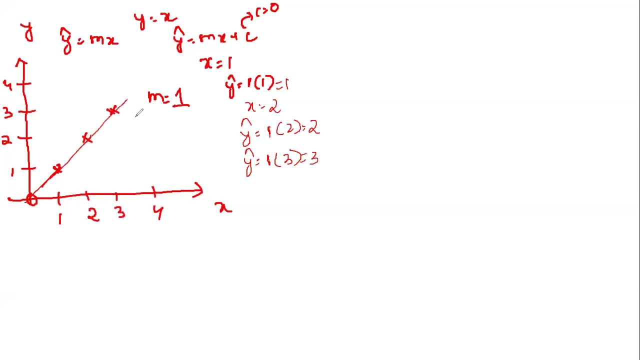 actually be 3, so it will pass through this particular point. now, this is what my best fit line is. you know, my best fit line for this particular value, when my slope is 1, when my m value is 1. very important now, after i get this particular equation, i will 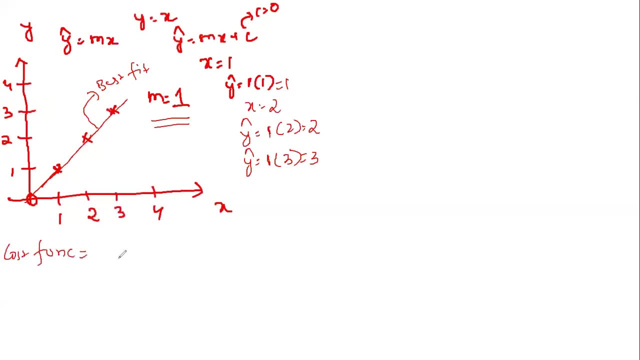 basically find my cost function. guys. remember i have already discussed about the cost function and the formula is something like: 1 by 2 m, summation of 1 to m, y hat minus y whole square. so this particular value i have to reduce it. you know, i have to find out this error. 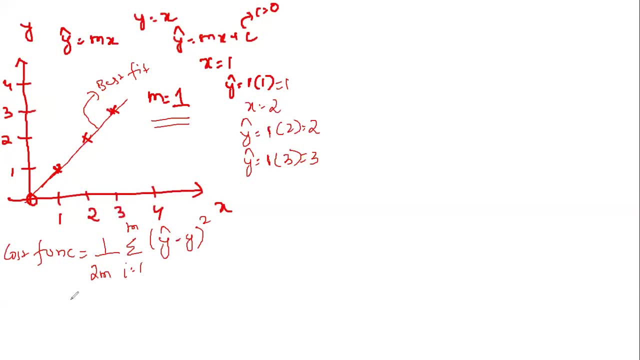 and try to reduce it. sorry, uh. now what i'm going to do is that i'm going to equate this term and i'm going to apply this proof: hundreds of Family Y values which can be assigned through expectation. no, your solution is going to actually be 2 plus 2 times the speed, which is going to be 3 times. that means i'm going to 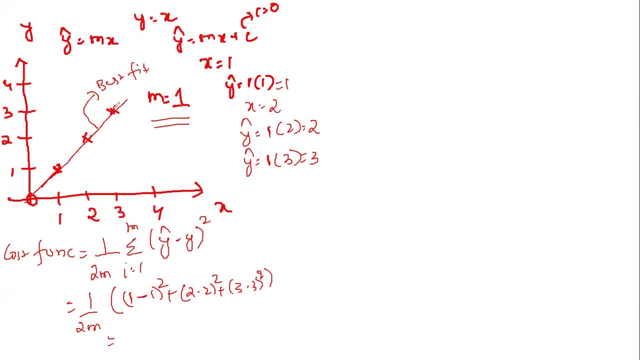 actually use the m value, which is three points, as my m plus 3 is equal to m. divided by m minus 3 times, that is what my m value will be. andHAHAHA111 bud by plus two. whole square is equal to m equals to m. M is m minus three points, so m equals to 2, so M equals to m is equal to m. 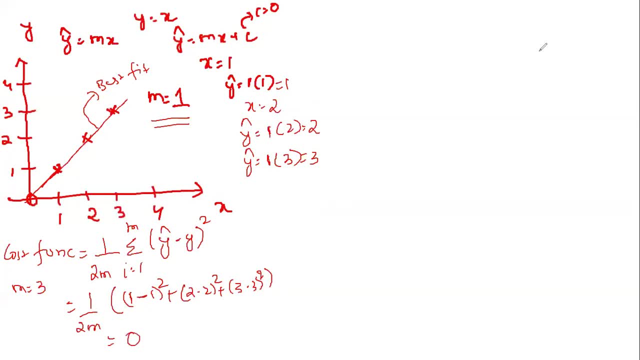 all right, surprised in all that. so this effective way, and, of course, for the summation, first of you know, one by six multiplied by zero is nothing but zero. Okay, So now this is very, very clear: When my M value, when my slope was one, you know, and for this point I got the 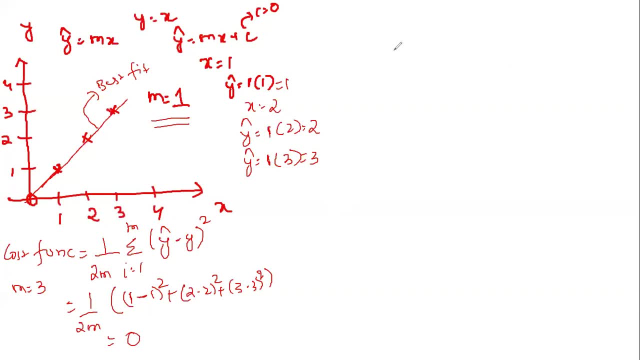 cost function as zero. So what I'll do is that I will try to draw one more diagram, And this is the most important diagram. guys, please focus into this. So here it is: I'm having 0.5, one, 1.5, 2.0, 2.5.. Right, And suppose this Y axis basically indicates my cost function. 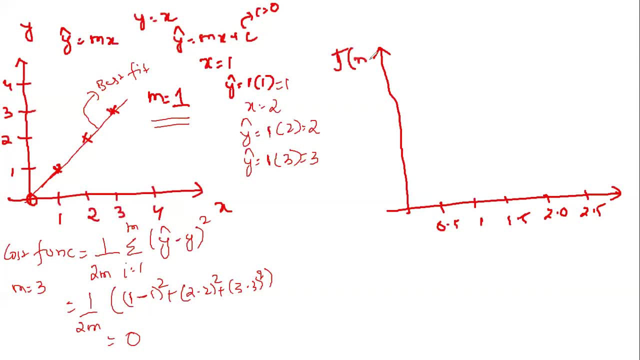 my cost function. Suppose I write it as J of some M value slope. Okay, And my, here, my slope is basically my M value, And here also I will write it as 0.5,, 1,, 1.5.. Now 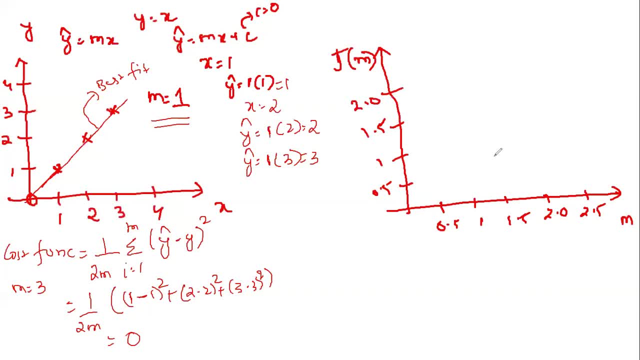 what I'm trying to do is that everybody please focus into this. What I'm trying to do it in in this particular thing is that, with respect to every M value that I've initialized, what is the cost function that I've got? I'm going to plot it over here Now, initially here, with respect to the M value as 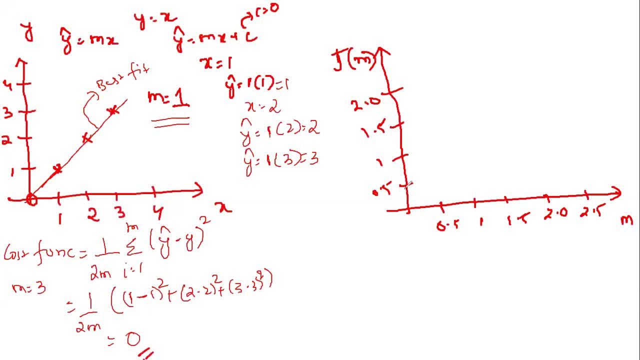 one. you know, I have got my cost function as zero, So what I'm going to do? my M value is one over here. My cost function is zero. So this is the point that I'm going to get. I hope it is. 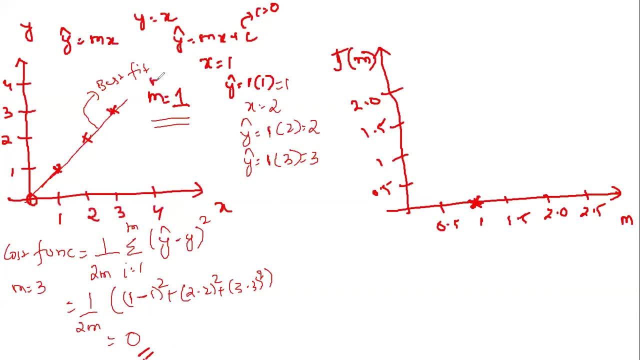 pretty clear Now, in my next step, what I'll do. I'll change this M value. Suppose I take my M value as 0.5.. Okay, Now, with respect to M is equal to 0.5 for this equation, if I equate. okay, my Y hat for X. 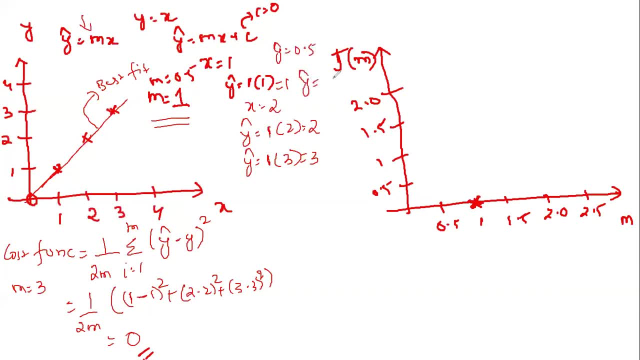 is equal to one will be 0.5.. My Y hat for X is equal to two will be one, And my Y hat for X is equal to three will be 1.5.. See how I'm getting this, guys. You just have to equate this. See when. 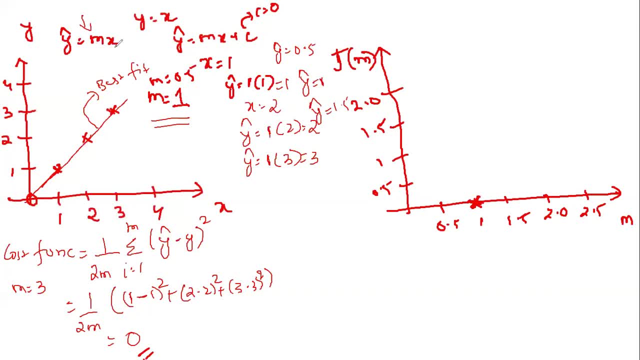 my slope is 0.5, when my X is 1.5 into 1.5, right, My Y hat is one, one into one one. Then when my slope is 0.5 and my X value is three, you know, three into 0.5 is 1.5. So I will be getting new. 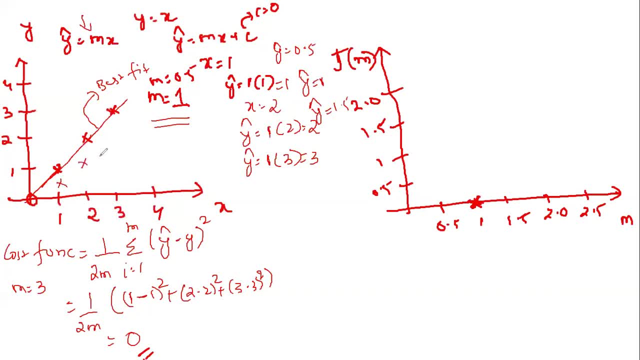 points somewhere like this: One, two and three. So this is my- oh sorry, This is my 1.5.. So when I draw my best fit line, it will look like this. You know now when I try to find out the cost. 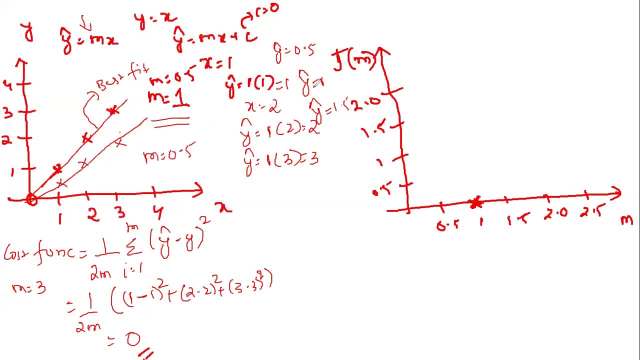 function when my M value is 0.5, you know I will be getting. you just have to equate in this Summation of: I is equal to one by M, and it will be nothing. but suppose my for X is equal to one. 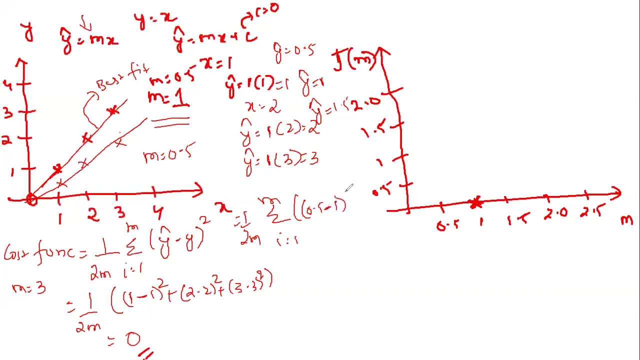 my Y hat was actually 0.5, 0.5 minus what was my Y, It was one whole square plus. similarly you'll do it for one one minus two whole square plus 1.5 minus three whole square, So just equate. 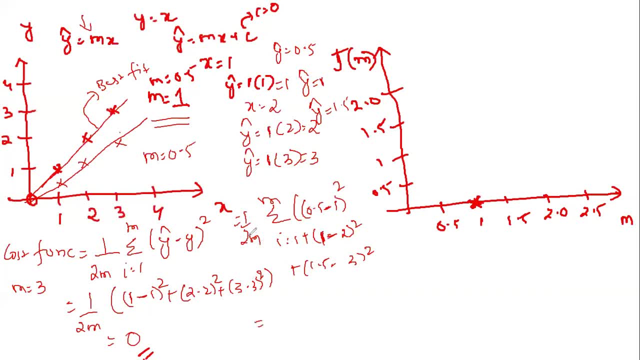 in this particular equation, place the M value as three, and M basically means over here. M is nothing but, or you can just write it as N, if you are getting confused. Okay, So N is basically the number of points, Okay, And if I, if you compute this, you'll be getting somewhere around. 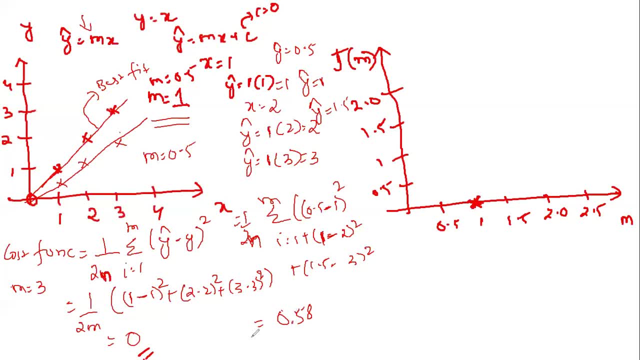 0.58.. Now when I say 0.58, you know this is your cost function. When your M is 0.5, your cost function is 0.5.. So here you can see: my M is 0.5, your cost function is 0.58.. So it. 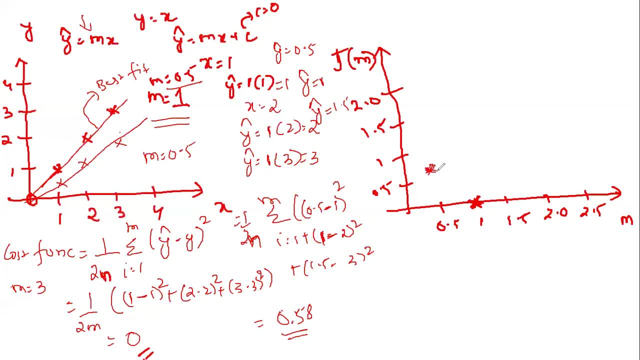 will be coming somewhere here. Your next point will be coming somewhere here. You know, then, different M values. you know you'll be getting points which will form this kind of curvature, this kind of curvature for different, different M values. you know, and when you draw this, 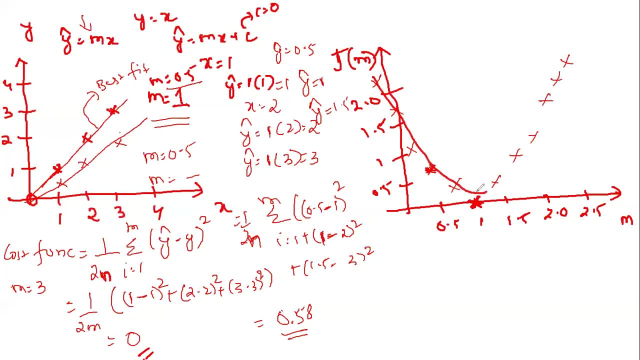 when you draw this, you will be getting a diagram which looks somewhere like this, which looks somewhere like this, And this is basically called as a gradient descent. Now, this gradient descent plays a very important role, guys, which I'm going to explain you in the next screen. Now, once you get this gradient descent, 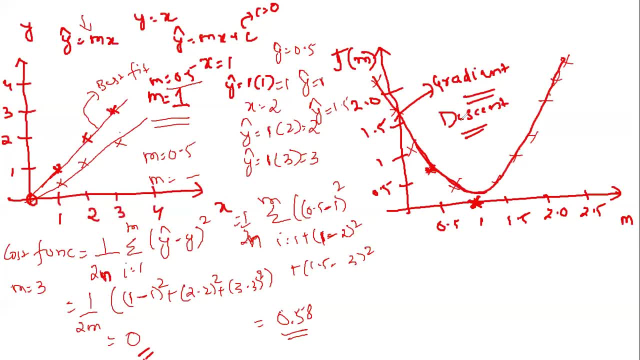 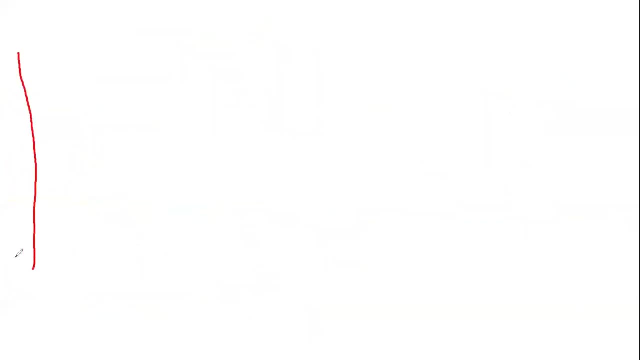 when should you know that you should stop, you know, for selecting a M value which looks good for this regression line or for the best fit? That is the next thing that I'm going to discuss. So before that, I'm going to clear all this diagram and let me just focus on two things. 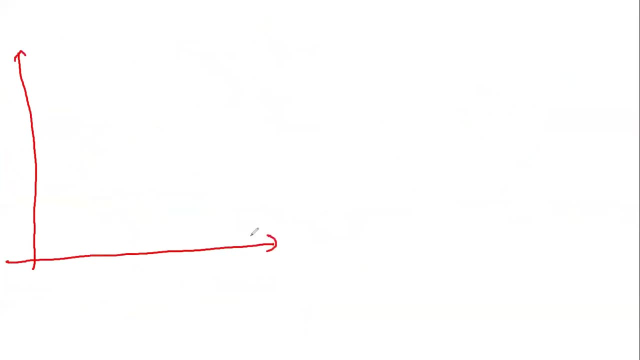 One is the gradient descent. As I said that, this is my M value, This is my cost function, That is A of M, And here I'll write it as 0.5, 1, 2, sorry, 1.5, 2, 2.5. Right. Similarly here: 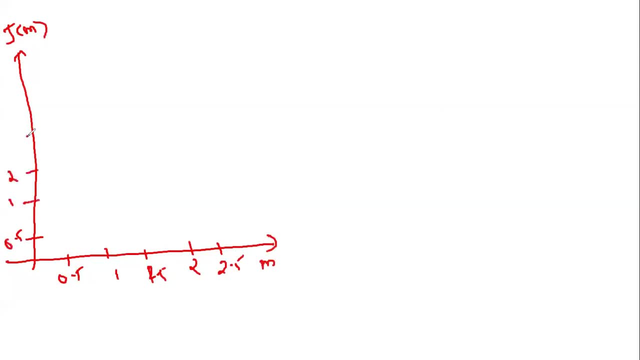 I'll write it as 0.5, 1, 2, 2.5, 3.. Okay, And you can see that my graphs look something like this. Just a second Okay. So my graphs look something like this: Suppose I'm getting this point somewhere populated. 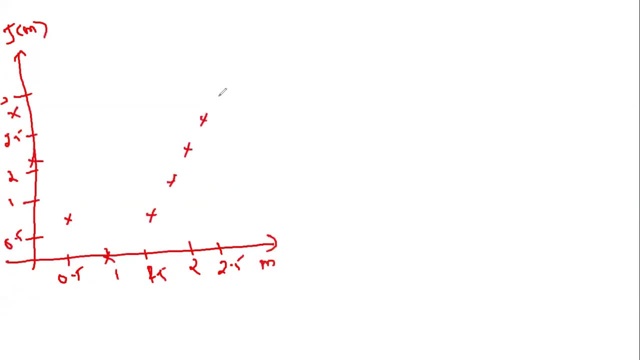 like this, and this point populated like this. I'm just going to draw my gradient descent. Again, it may not be approximately correct, but I okay. sorry It may not be approximately correct, but I'm just trying to draw this diagram properly for you, Okay. So here it is. 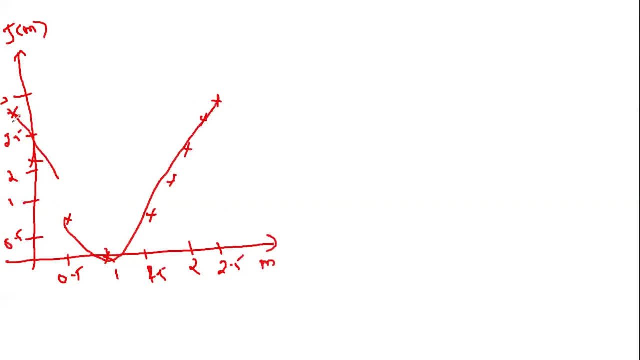 I'm going to draw this, which looks like this and which looks somewhere like this: Okay, guys, So this is basically my gradient descent, which I've drawn again. I'll write it as gradient descent Now. in my previous diagrams that I've already shown you that, based on different 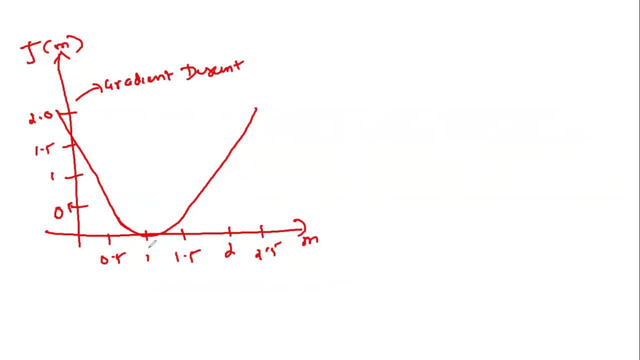 different M values, we're getting different, different points And, finally, we could follow this particular structure. But uh, the next thing is that how do we arrive to this particular region? And this region is basically called as global minimum, Global minimum. Now, the next thing is that I need to arrive at this particular position. 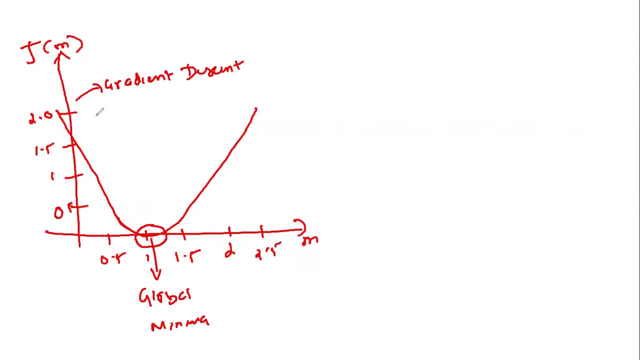 So for for that, initially, suppose I consider that based on some M value. I got my initial point somewhere over here, you know, somewhere over here. So when I got my initial point over here, that basically means that I have to move downwards, right. 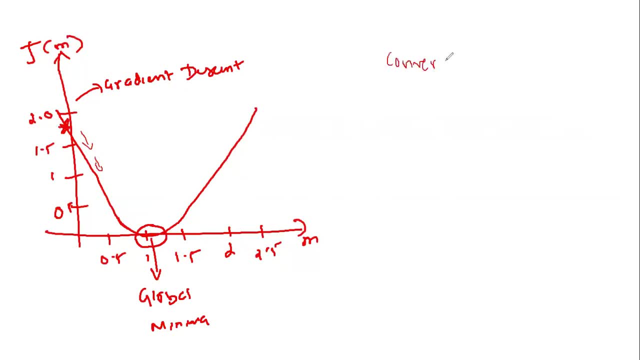 So, in order to move downwards, I will basically write a theorem which is called as convergence theorem. Okay, Now for this. convergence theorem basically says that the M value you should subtract with M minus derivative of M. you know derivative of M with respect to M. you know derivative of M with. 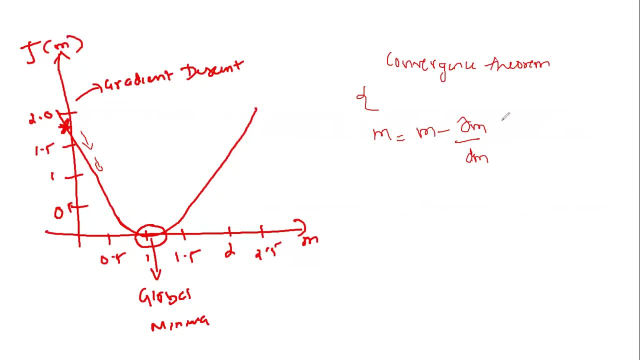 respect to M, such that you know, this derivative multiplied by one more value, which is called as learning rate, which is called, which is basically indicated by alpha. So this is my learning rate. Okay, Now let me just show you why this. 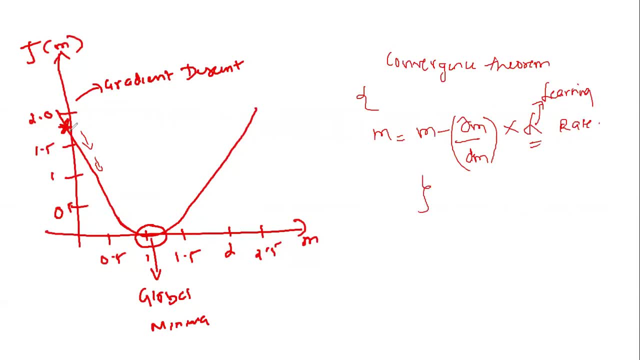 particular equation works. Okay, Now, suppose initially, and this derivative is basically my slope. Okay, This derivative is basically my slope. Okay, Now let me just tell you. now suppose for some, for some M value, I got to this particular point or at at particular 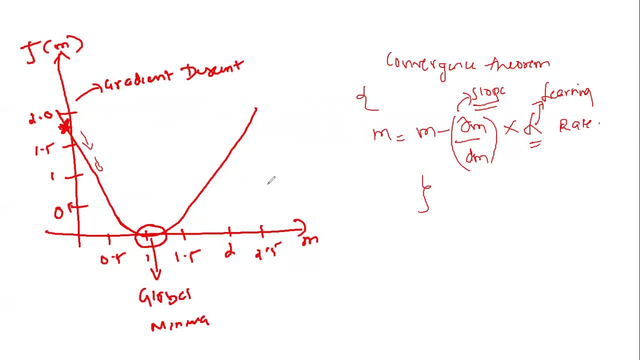 of this position and then I'll be applying my convergence theorem. Now, convergence theorem basically says that I have to subtract with the slope of this particular, of this particular point. So if I want to find out the slope, you just have to draw a straight line like this: 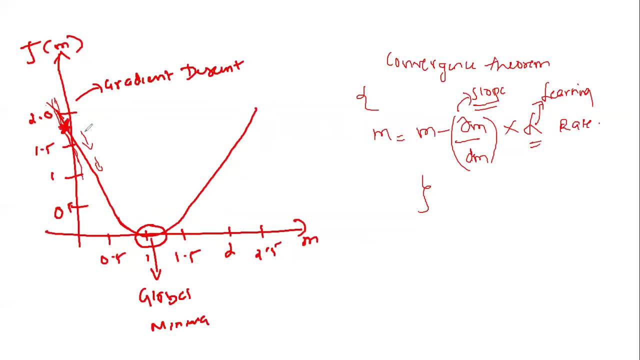 Okay, And this particular straight line is basically helping you to find out the derivative of the slope. When I draw this particular slope, the next thing I have to find out whether this is a positive slope or a negative slope. That is important to find out now. how to find out whether 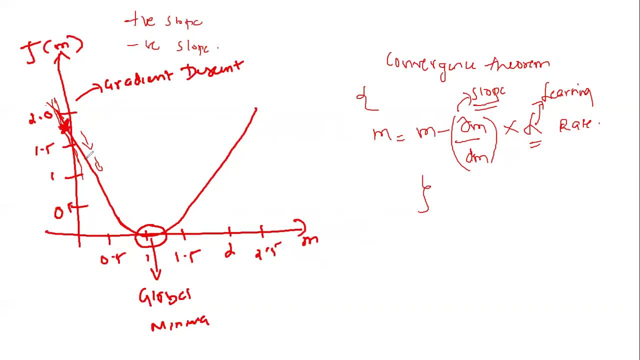 this is positive or negative. Now you should see or focus on the right hand of the slope and the left hand of the slope. If the right side or the right hand of the slope is pointing downward, you know it's pointing downwards. At that time you can say that this is basically a negative. 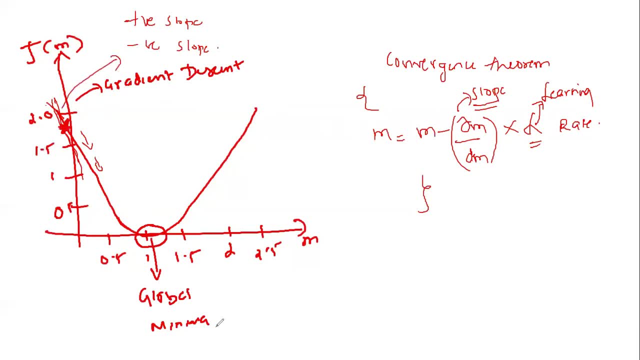 slope. You know the negative slope. Now you can see that at this particular point, suppose my M value was somewhere like minus 0.5.. Okay, Then your feasible M value is somewhere around one. Now, when you find out your negative value, your, your, uh, this particular point value is having. 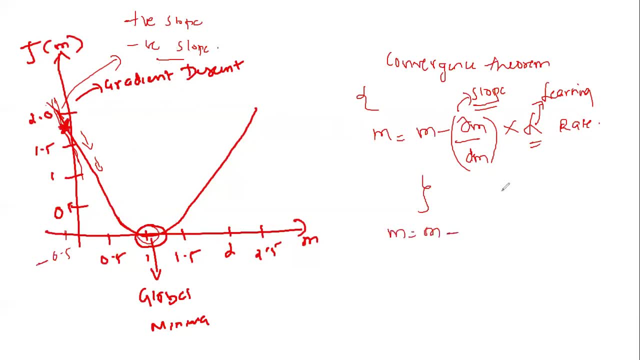 a negative slope. What you do is that you subtract M with some and then, whenever you do a negative slope, you subtract M with some, and then, whenever you do a negative slope, you subtract M with some, and then, whenever you do a negative slope derivative, you'll be getting a negative value. 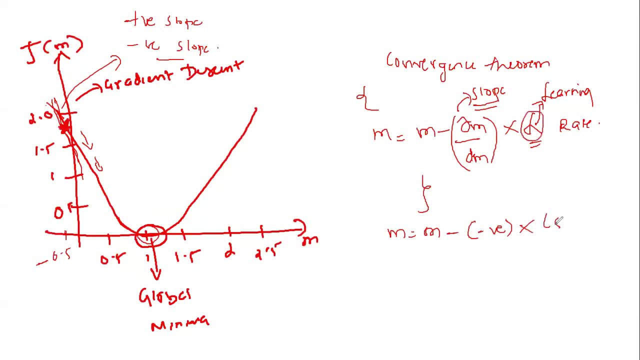 Okay, And this alpha or learning rate will be a smaller value. I'll tell you why we have to select this as a smaller value. When I say smaller value, then this value can be somewhere like 0.001.. Okay, So when I take a negative slope, okay, When I find out the derivative of a negative slope. 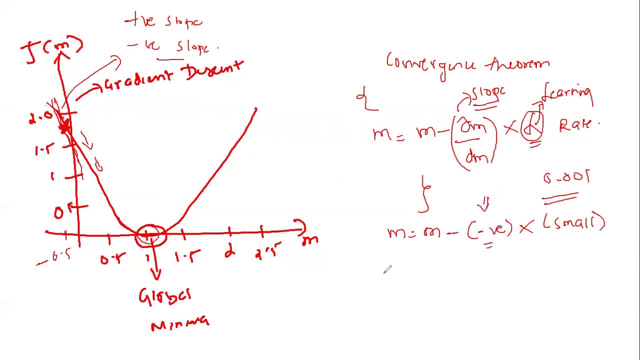 then it will be a negative value and which it will be a very minimal or small value. Okay, Now, when I do like this, I'll just write it as M plus some positive value. you know, a smaller positive value, because see minus into minus is plus right. So plus positive, smaller value. 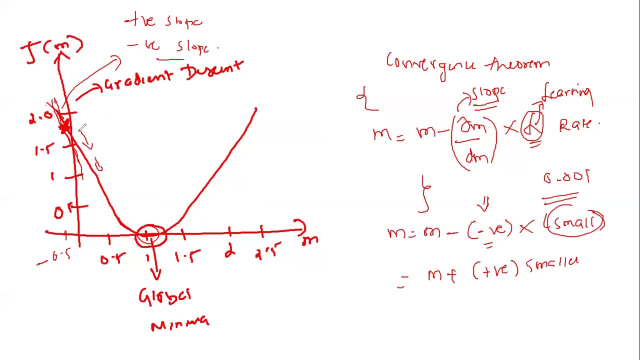 because this is a smaller value of learning rate. So what will happen is that that basically indicates my M value should increase for minus 0.5 and it should come nearer to one. So this step will be very, very small. You know it will be very, very small And as iterations and different, 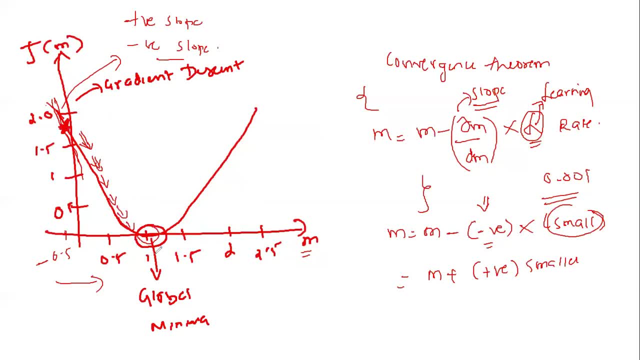 M values get selected, this will be moving towards this particular global minima point. Now the the next thing is that if I select this learning rate as a larger value- like one- okay, 1.00,, what will happen is that, instead of taking the smaller step, 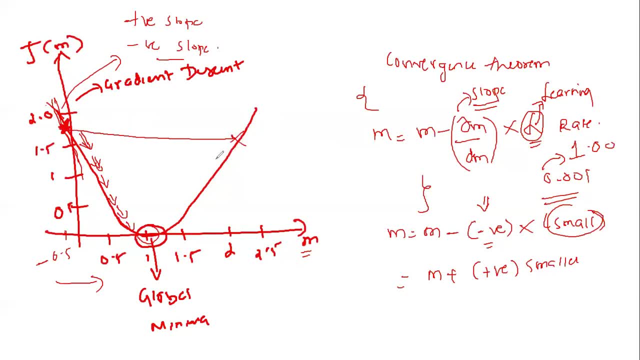 this point may jump to some other points like this: Okay, This may take a longer jump and it may not reach this global minimum. even after many iterations. even after many iterations, it may not reach this global. So for that reason, we usually select the learning rate. 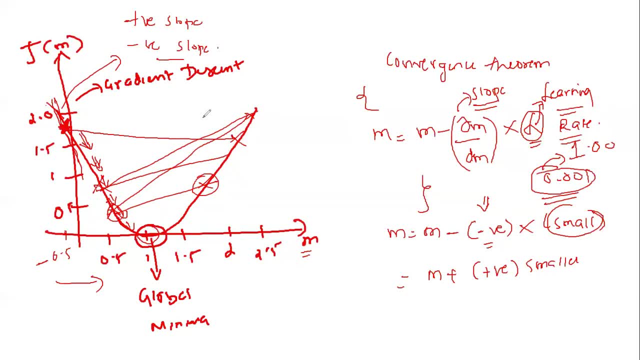 value as a very smaller value, you know. And okay, Let me just consider that Suppose, for suppose I, I, I selected a random M value and I got the point somewhere here. Okay, Somewhere here, supposed it. I got it somewhere here. Now, you should see that when I get this point over here, 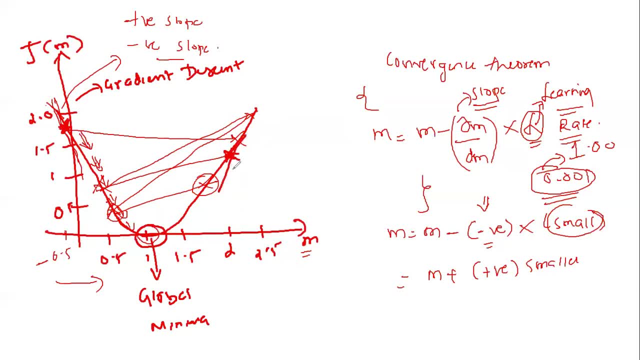 if I try to find out the slope of this particular point or the derivative of this particular point, I'll see that my right-hand side is pointing upwards on my left-hand side is pointing Speaker 1, So this is basically my positive slope and when i find trying to find out a derivative of a positive slope, this basically: 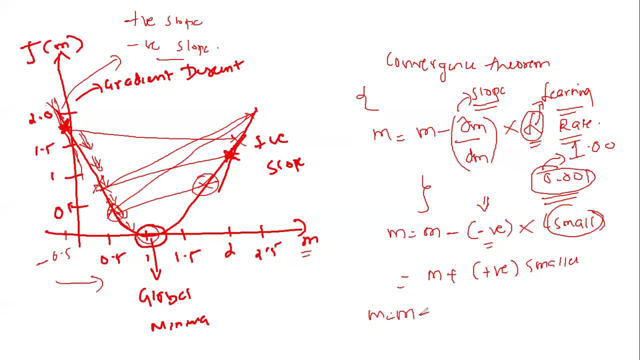 indicates that my derivative will be nothing but m minus. this derivative will basically be a positive value and then i'm going to multiply with my learning rate then, which will be nothing but m minus some smaller value. when i do m minus smaller value, then you can see that initially. 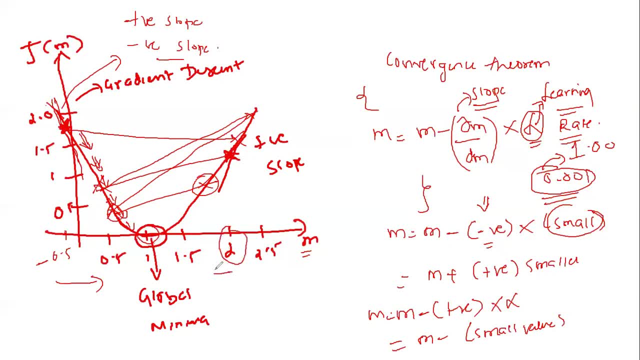 suppose my m value was two, i have to reach it to one, so it will subtract a smaller value and we will be moving in this particular position. so always, it is very important to understand that our, our learning rate should be very, very small, and this convergence theorem is very, very important. 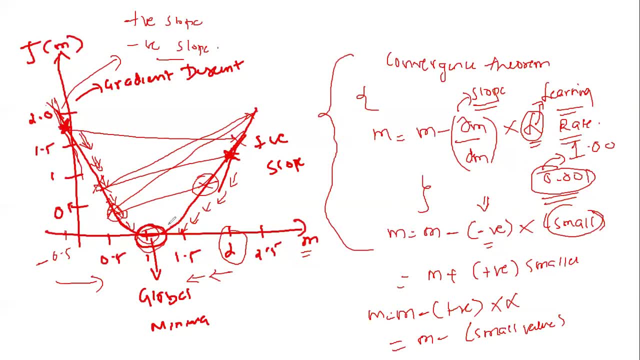 to reach this particular global minima point. so as soon as it reaches over here, at this particular point, if i try to find out the slope, the slope will be zero, the slope will be zero, and when i have a slope is zero, that time my m value will actually my m value will specify that this should be the value. 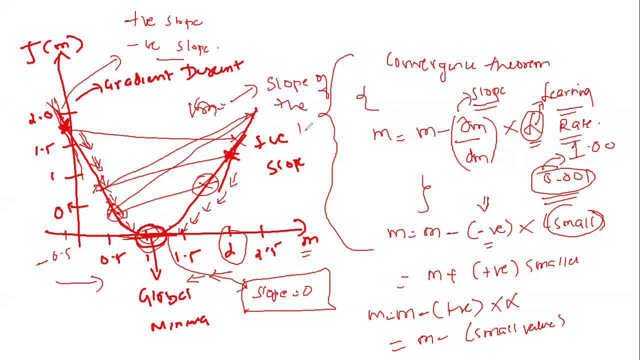 or this should be the slope of the best fit point, best fit line. until then, i have to follow this convergence. so once i am a, once i get to this particular point at this particular location, when my slope is zero, i will basically- or my algorithm will basically- be considering this. 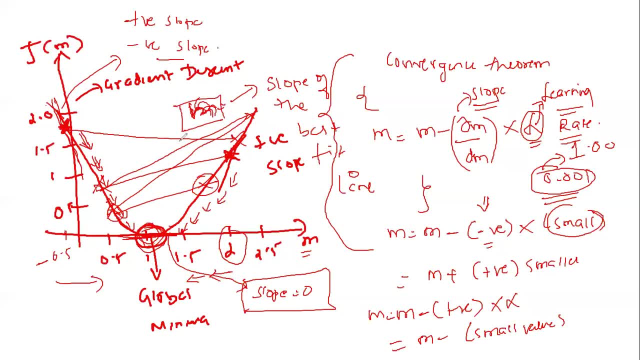 m value as my best fit, as the slope of the best fit line, and that is the point where i have to stop training and that is the point which will be able to determine that that is the value of my best fit. you know, and this basically indicates the whole, 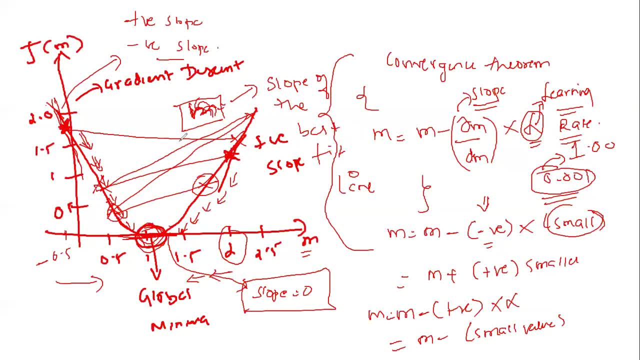 uh explanation, the theoretical concepts, along with maths, of the whole linear regression algorithm. now the next thing is that if i have multiple multiple features in uh suppose, if i i just i don't just have only one independent feature, i have multiple independent feature at that particular point of time, my gradient descent will look like a three-dimensional gradient descent and i will be 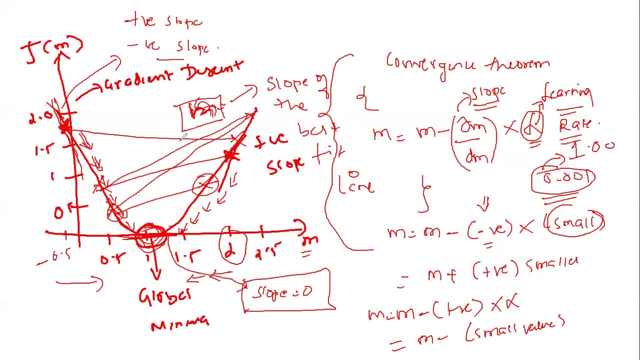 able to draw a 3d diagram or a 4d diagram based on the number of features, and each and every feature will try to move towards the global minimum point, which will be this particular minimum. i hope you like this particular discussion guys. i hope you like the step-by-step process and how we derived. 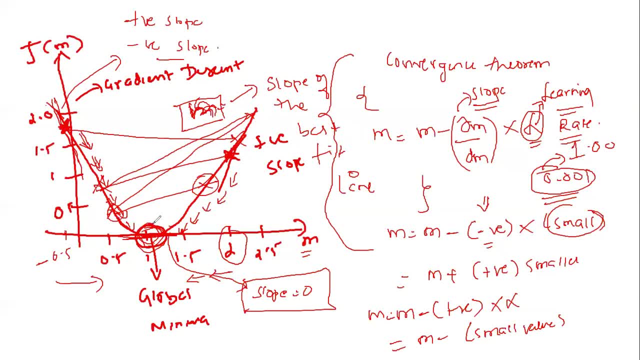 it. please go through this video from once again, from the starting and now, after understanding this thing, how do you implement it? i'll be providing the link. uh, you can see in the top right corner, i'll be attaching a link and there you can actually see the link, and then i'll be providing the link. 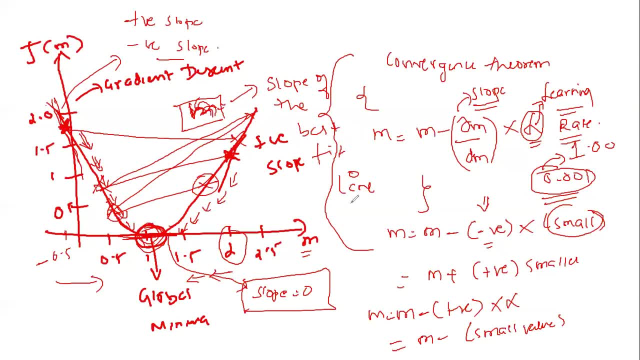 and there you can actually see the link and then i'll be providing the link and there you can actually see the implementation part of simple linear regression and multiple linear regression. i hope you like this particular video. um, please do subscribe the channel if you have not subscribed. 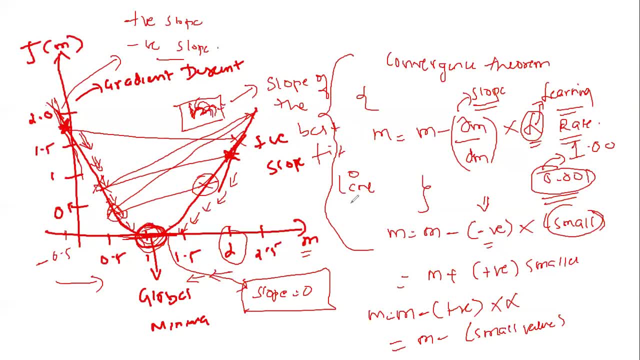 and, yes, i'll be coming up again with some new, uh good videos where i'll be discussing all about this- mathematical combinations, and we'll i'll try to derive all the things in front of you, okay, so, uh, god bless you all. uh, keep learning. you're doing a great job and thank you for. supporting my channel. thank you, one and all. have a great day ahead.